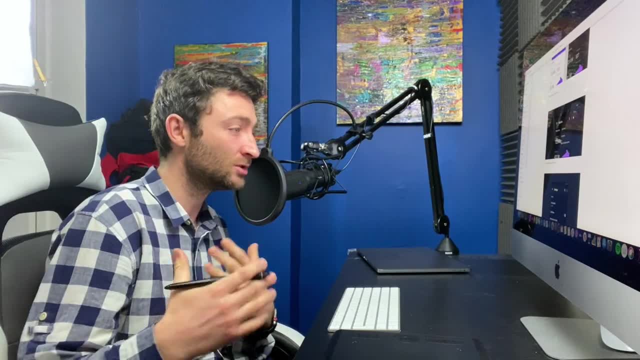 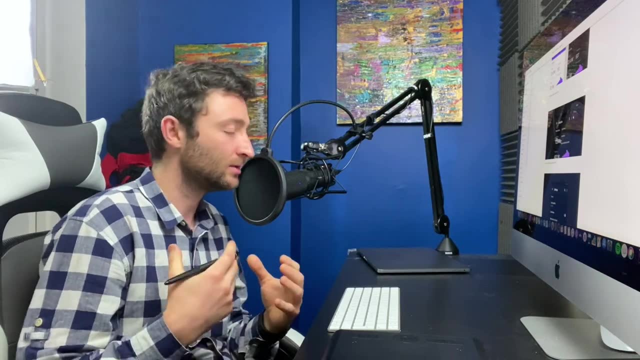 waste time really in reinventing the wheel on things just to be a designer. But a lot of things. a design thinking rather than design application. So you should be thinking about the user flow, thinking about how your app works. You need to understand material design as a designer. 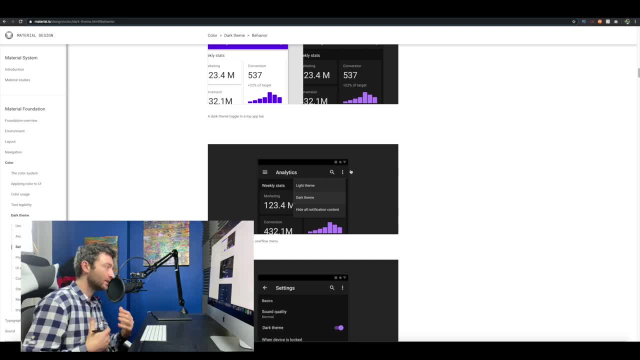 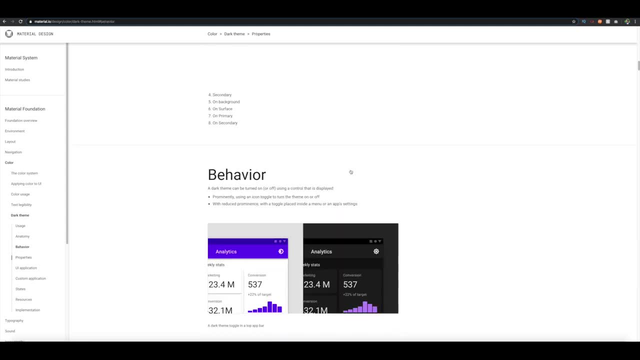 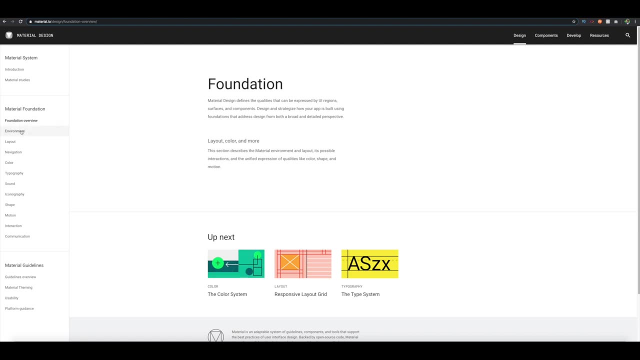 And then the outcome is actually quite quick. But all of that knowledge gain takes time. by reading stuff like this- And you know, by you checking out this overview, it's a good introduction to it. So we can- we can- have a look at what the foundation is first for material design. 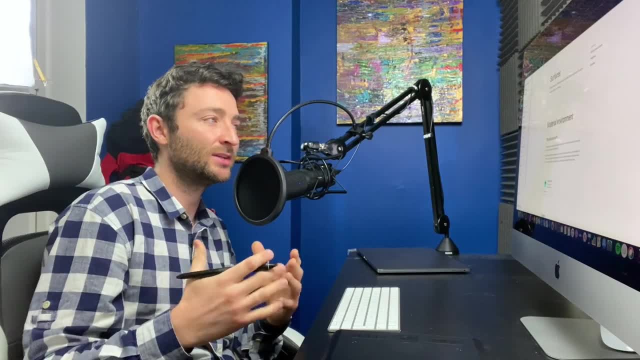 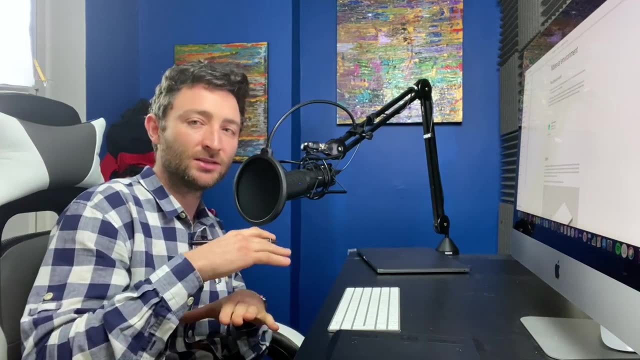 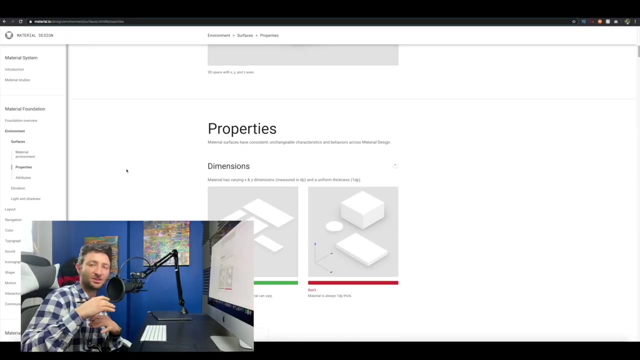 and how it's how the whole thing works. So I'm going to go ahead and show you a little bit of the whole thing is based is it's based on real world, real world physics, So a lot of it is to do with depth. So there's different layers on on the applications and those layers cast shadows. 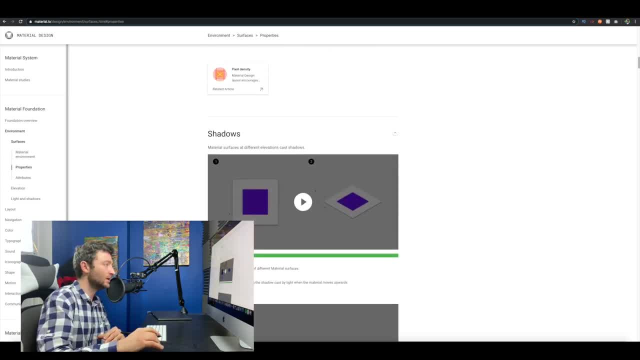 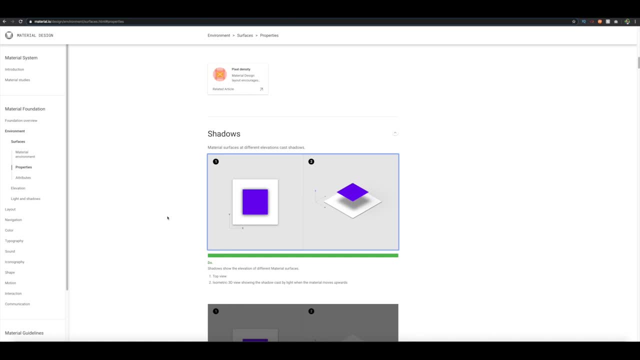 So it's not 3D, but it's. it's more like drop shadow ish. If you go in here, you can see how, when things are elevated and on layers above other things, the shadow acts like it doesn't work. So it's a little bit different. So it's a little bit different. So it's a little bit different. 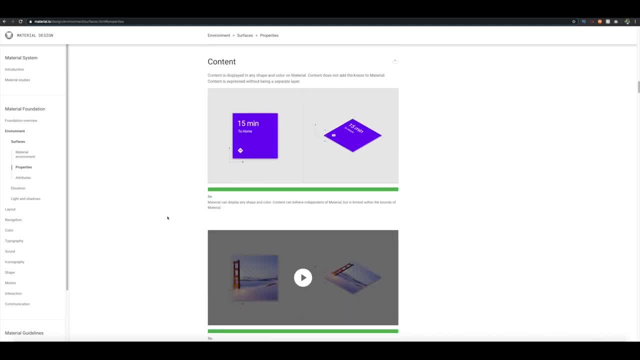 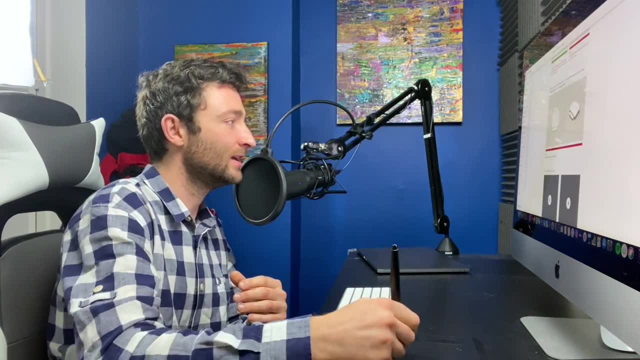 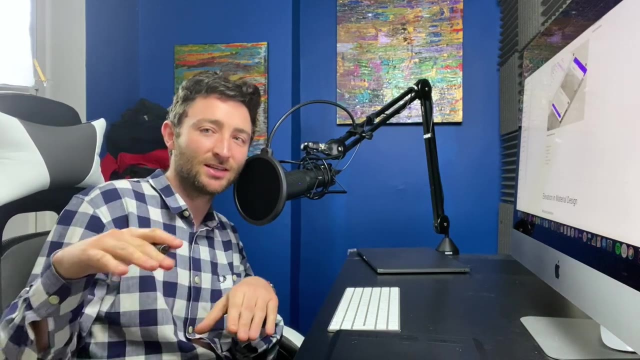 They did a lot of research into this And it's something that you really need to understand: all the do's and don'ts about how things are on in the physical life here. Then they talk about elevation and how you know when something slides over something else, like a menu slides in all of 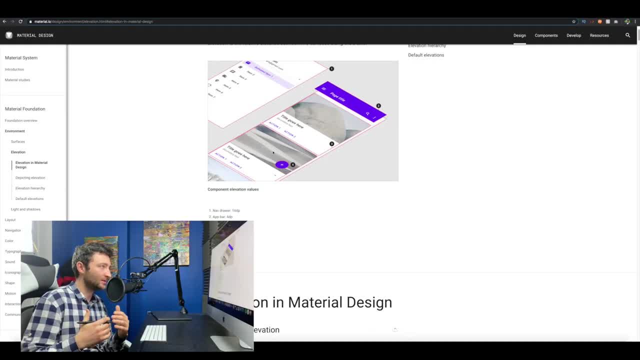 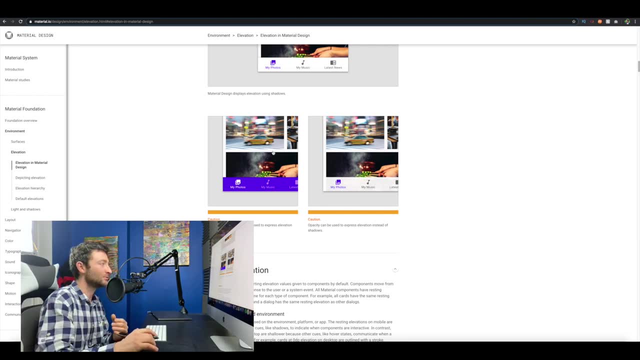 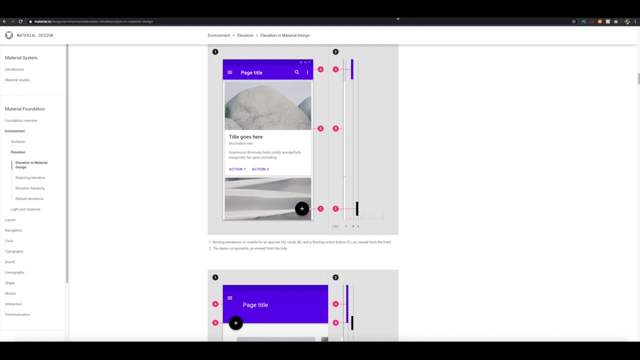 the shadows come into play and it's it's kind of like science in a way. It's all they're doing is mimicking the real life, And whenever you're designing something for Android, you should really check it out. And before I say that, if you want to develop for Android, 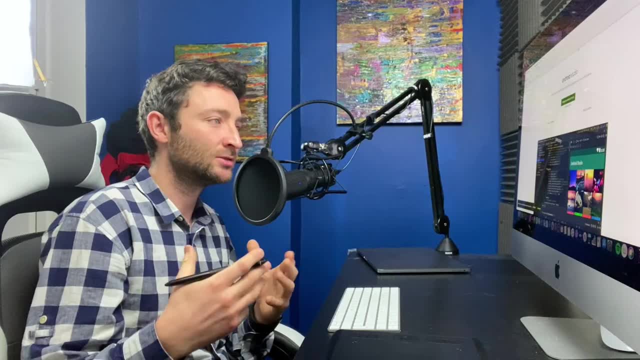 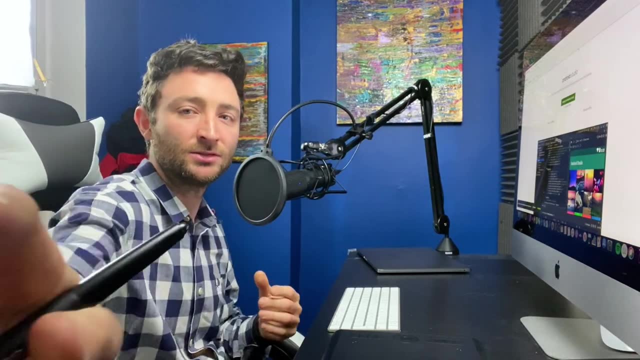 check out Android Studio: developerandroidcom. It's something that you can take these designs that you do in whatever format you put them in. It's got a visual editor in there. If you know a bit of code, it's something that you can. it's something that you can definitely check out. 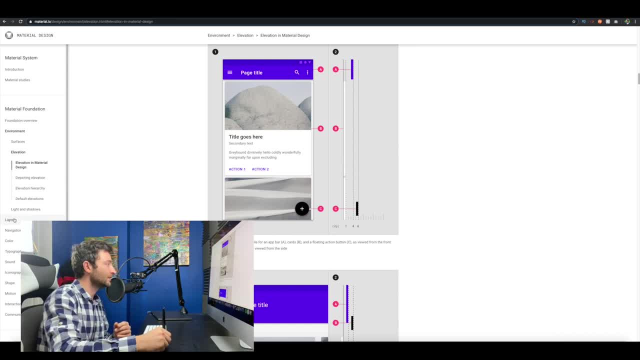 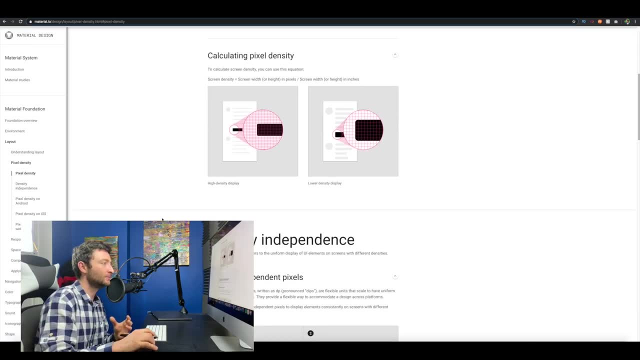 So that's developerandroidcom. Then if we go in we can have a look at understanding the layout, How the grid works, how the pixel talks about pixel density on different- there's different- resolutions of displays. it talks about how Android works. all that out. 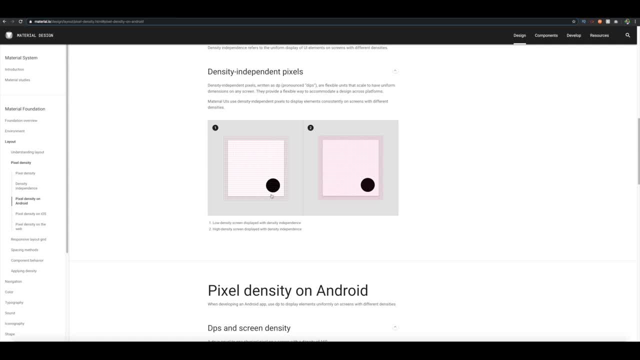 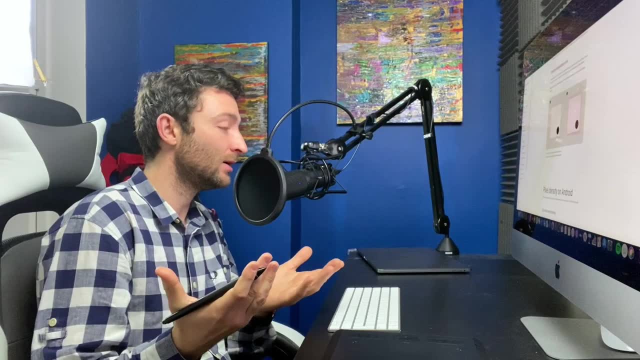 So you can see if you design something, it stays the same size on the different screens. That's something that Apple did quite cleverly. So I remember designing for the iPad one and then the iPad two came out and it was double the resolution of the iPad one. But that's something. 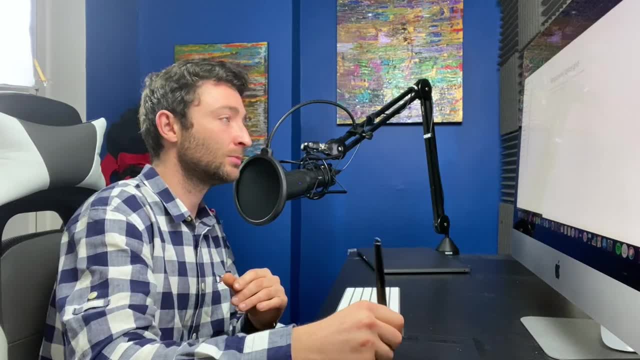 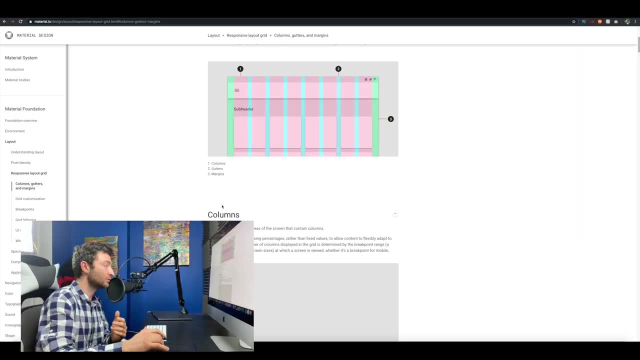 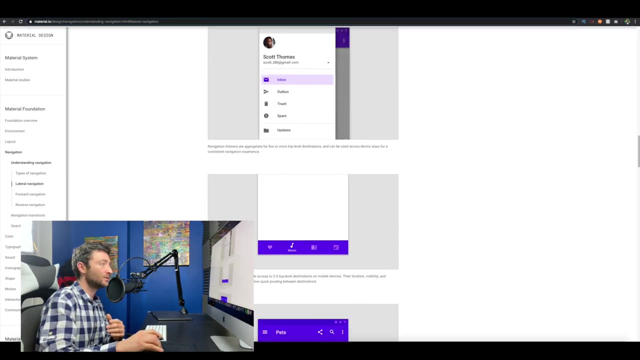 that Android have nailed here. Then they're talking about like responsive grids and how different the same app can work for a tablet or a mobile different sizes. So you've got your grids in here. Then Android talks about navigation And you know, you've got these slider menus. 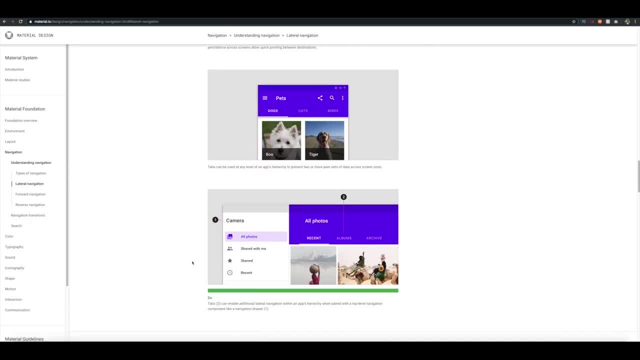 you've got bottom bar menus. don't reinvent the wheel here, because you just wouldn't be able to use it anyway. So understand how all of these different menus come together and create a beautiful experience. Then we have color. So we talked about the different colors. 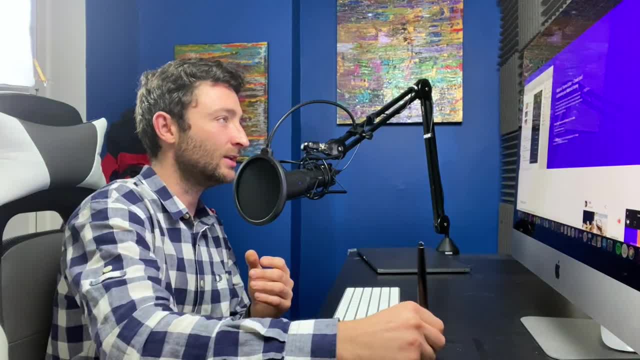 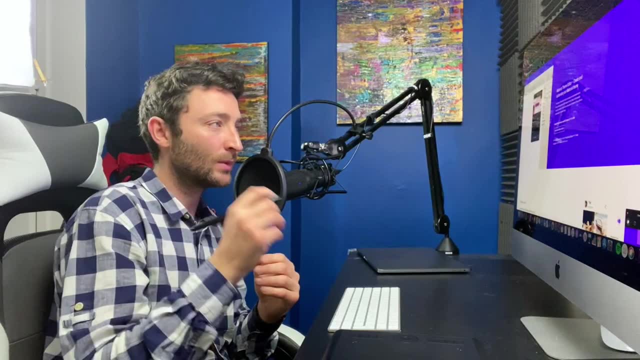 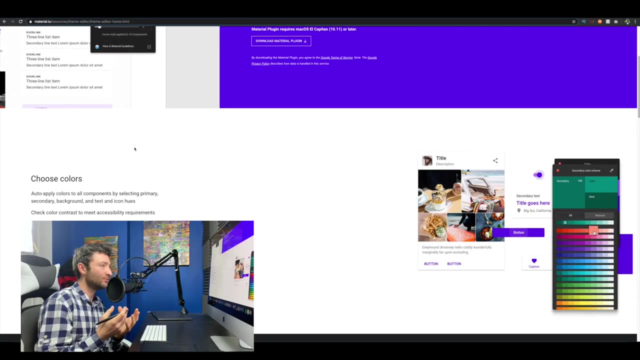 within Android Studio there's different places you can go, So they've got this theme editor as part of the resources. It's a plugin you can download for Sketch So you can put it in. you can put your own colors in and it helps shape the identity of you know of material design. 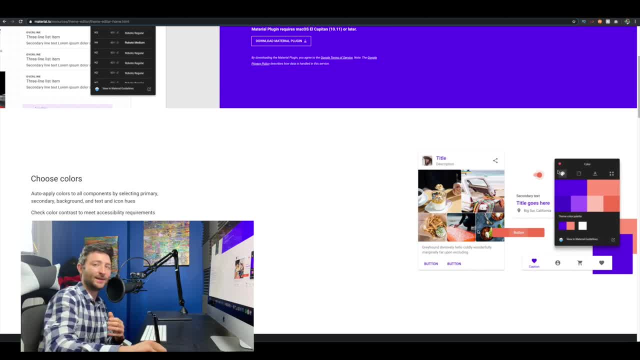 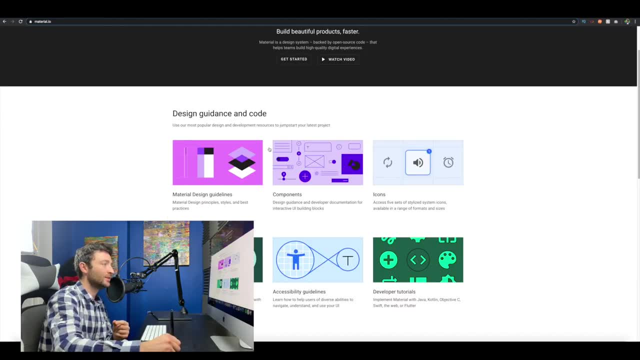 Like it's not. you're not all stuck to these greens and stuff that Google use, Like you can see here. changing the color palette changes the button and so on. Then you can check out the different color and color settings So you can see the colors that you want. 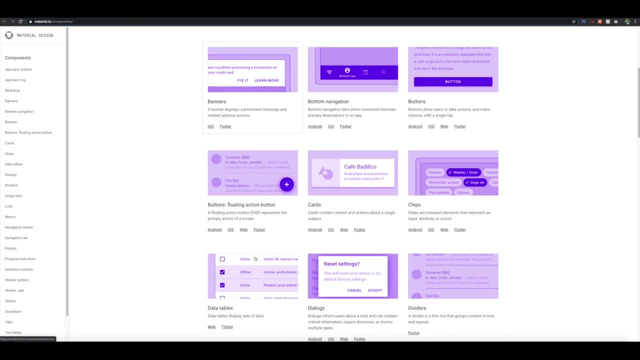 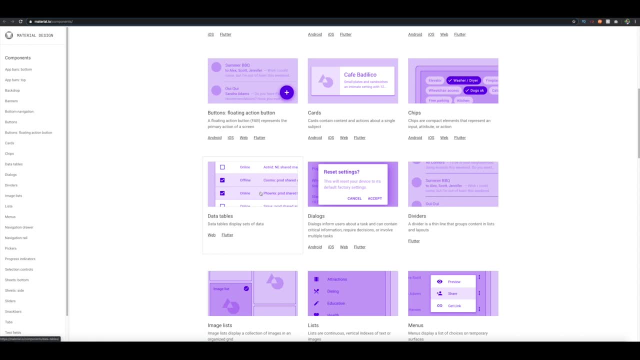 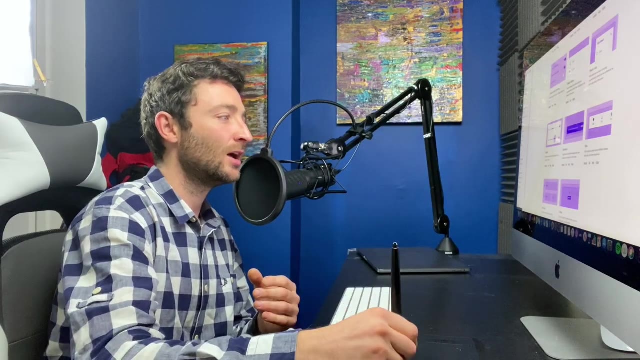 the colors of the components So you can see things like all these top bars You can see. you know you can see cards, tables. you know so much time I spend on figuring out tables when I've been working in companies before, and dialogue boxes, sliders, I mean, there's so much. 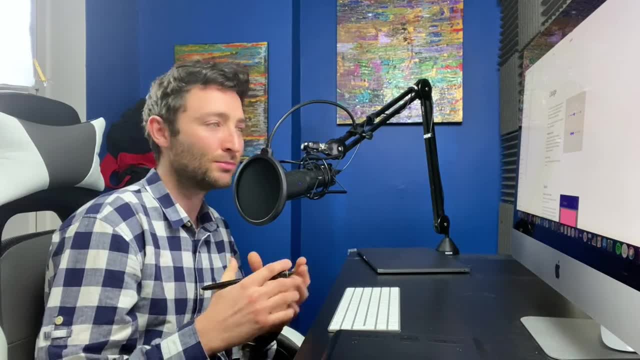 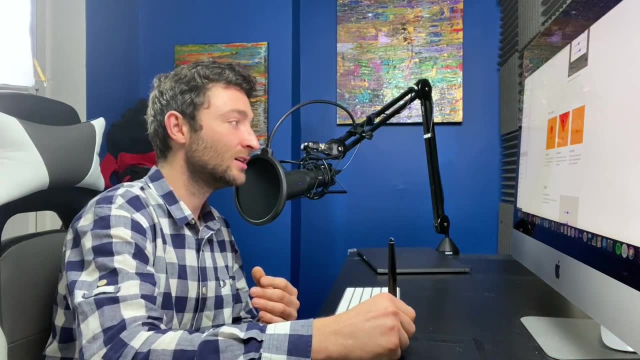 stuff for you to go in here and understand, And the fact that it's all been done for you is something need to spend a year making something like this was that is honestly the amount of time it takes figuring out things like menus and even simple things. 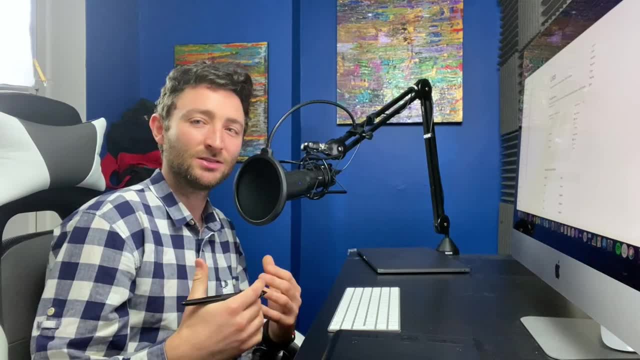 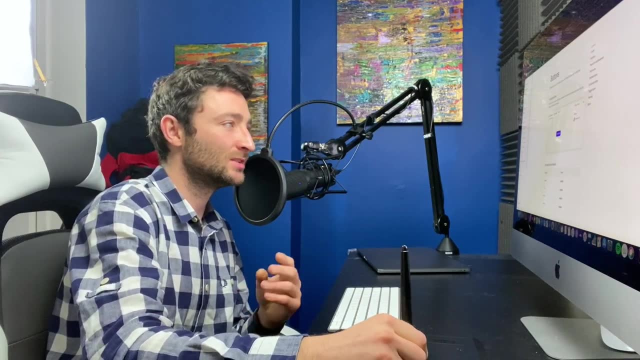 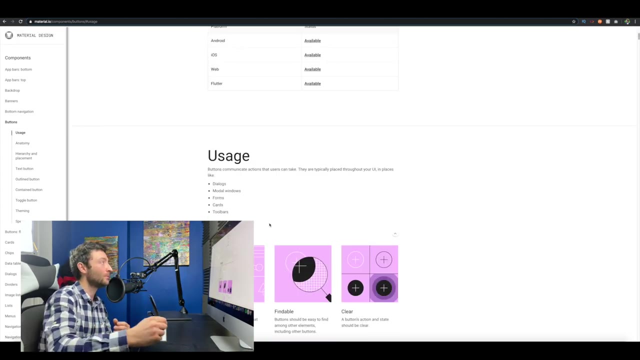 like lists, the amount of time that they've got into into doing research for it. make sure it works. you know buttons- they've got all the styles here and you know there's little. it's quite cool the way you can. you can change it here so you can see what it looks like with an icon or not. that's all in material. 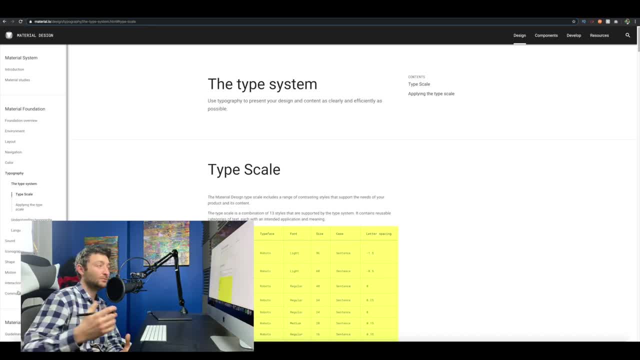 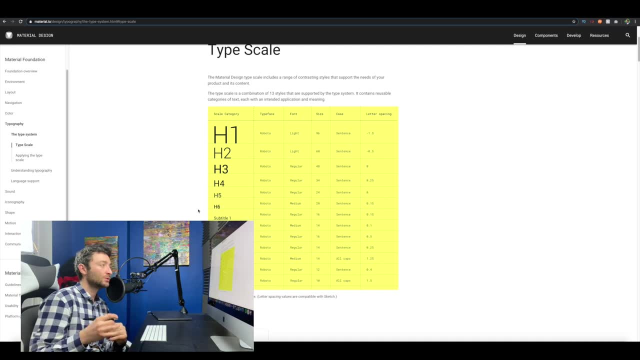 design, then it's got its own whole type system. so whenever you design something for a digital device you have type hierarchy. so H just means heading. you have heading one to six and that's just your main headings on a website. so for this you can see like these big titles are all probably H, H free or H to the. 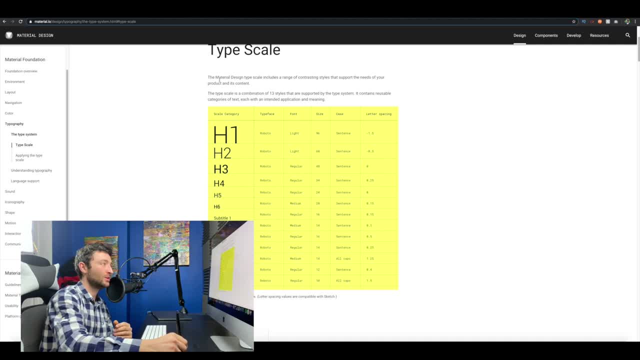 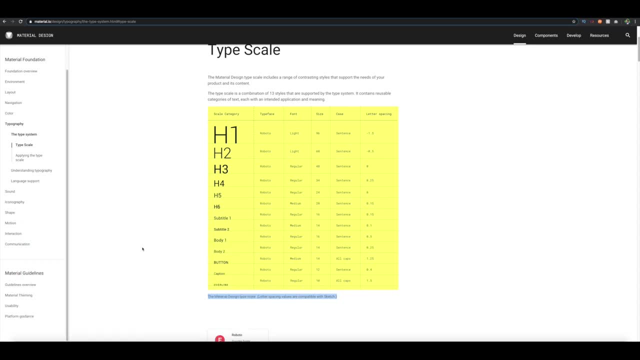 main title on your page is a h1, and then you have body copy here, which is the main font, then you'll have caption here, which is a smaller version, and so on. you just need to learn all these, all these different styles, but you can download the fonts that Google use from here. 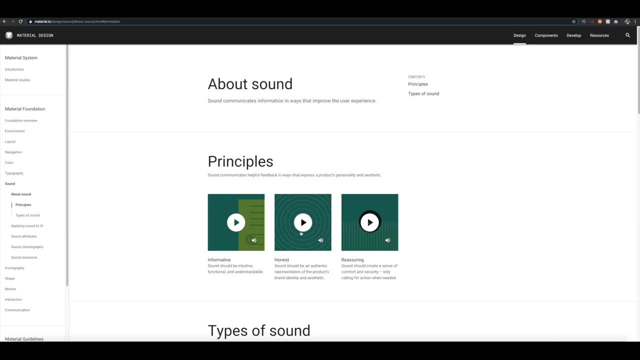 they've also gone in in this new release talking about sounds. so a little nice little dink. might be a little bit of Zelda, but nice little dink sounds. so you can. you can understand when to use sound on a website, never really use it as a. 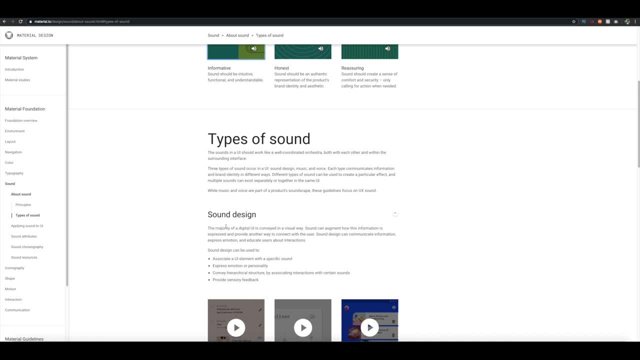 back-to-back. use it as a back-to-back. use it as a back-to-back. use it as a background. it's a bit too intrusive if someone's in work. they don't want French rap to be blasting out over the speakers like I did for a university. 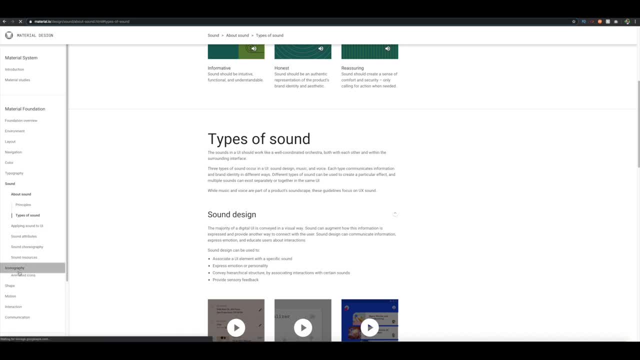 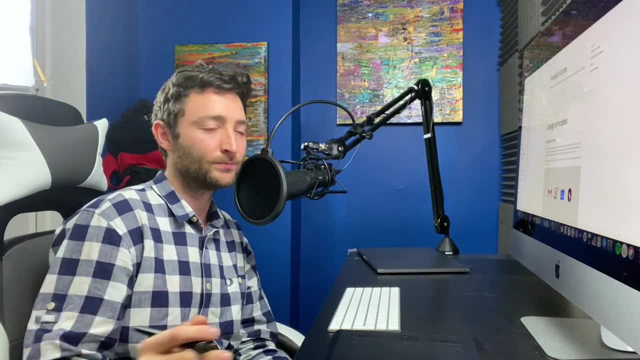 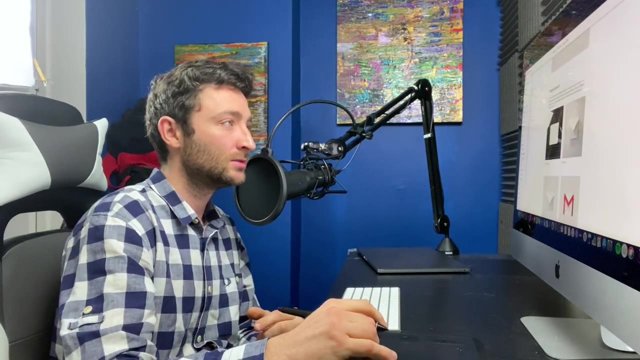 project once which, yeah, I'll never use sound again. but you know, if you add something to a cart, maybe you can have a sound which is a bit reassuring. there's a, there's a whole. you know there's a whole thing on designing little app icons. you know a lot of work goes into them so you might not think of by. 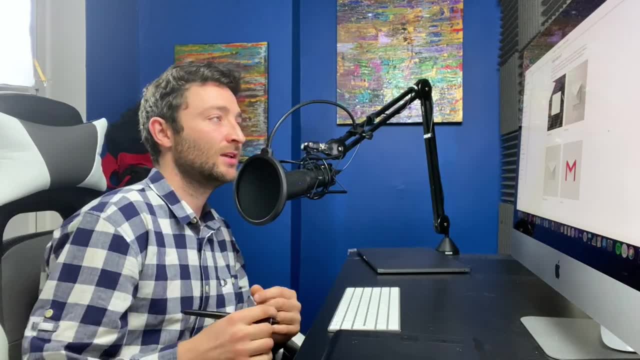 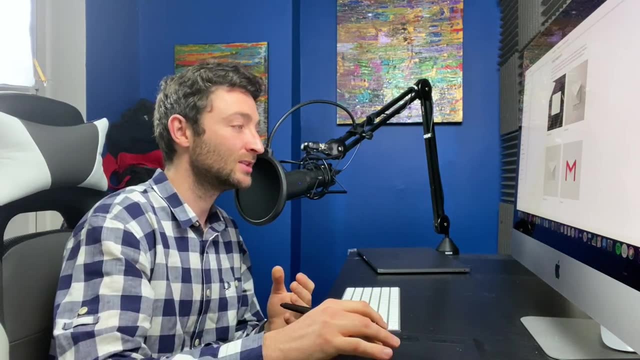 looking on it. but look at how this mail icon was made. first they actually did it in real life. then they looked at the lighting of it, because a lot of this- is it a lot of material design- is lighting. then they did this prototype and then they added color on to it, and that's how. 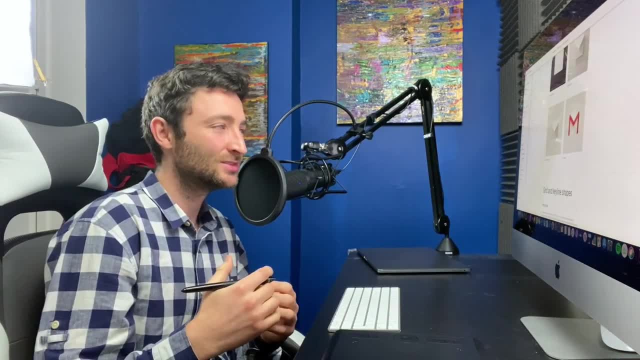 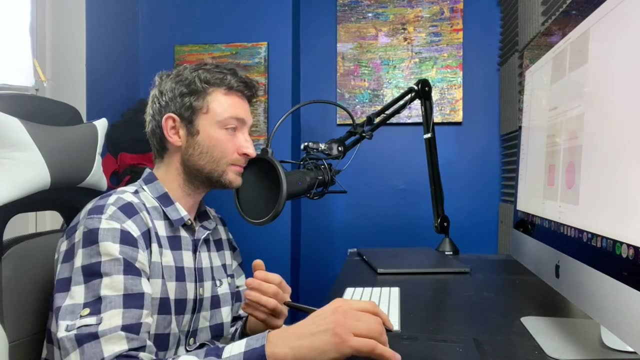 they got. that's how they got that design. so you look at anything, it looks simple, but it's actually not a lot of thought goes into it. and then here you can talk about how you can make your own design and different shapes to use where to put. 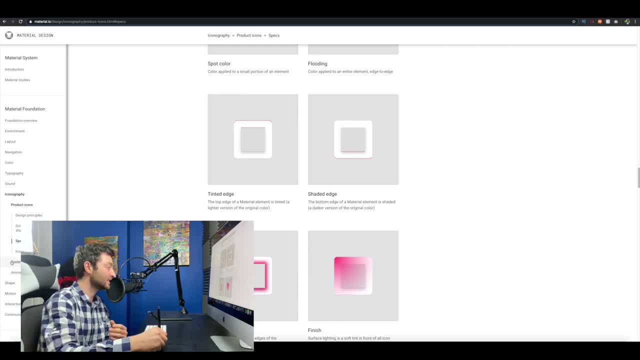 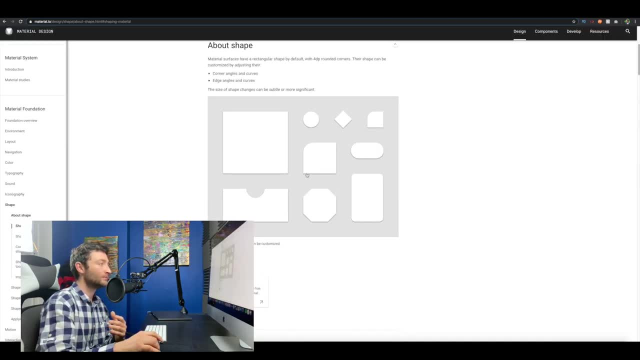 it. it's something that you need to know when you, when you're creating things like icons. you need to know when you, when you're creating things like icons, then you know there's all about how to work with shapes. you know different shapes can be used for different things, like this cutout here at the bottom. then 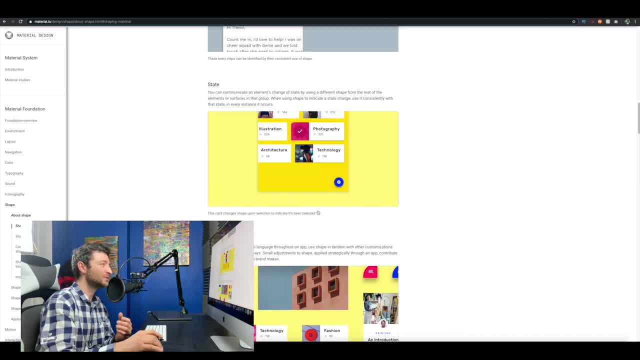 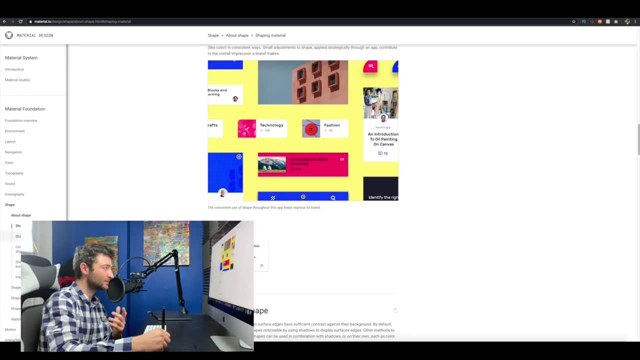 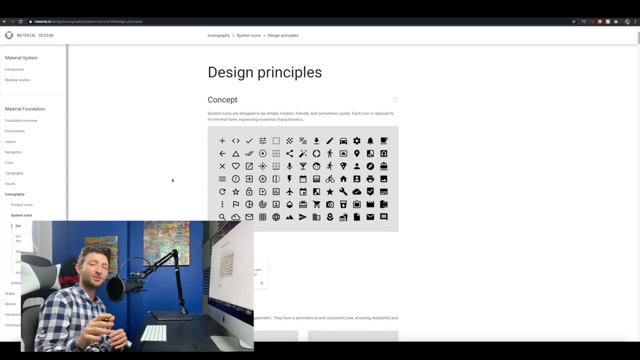 they have these. you know. it's just different shapes are used for different things. like this around the corner might be used to indicate someone's been selected or not, and they have a whole philosophy around there. you know there's iconography as well, so you've got all your system icons, so don't bother. 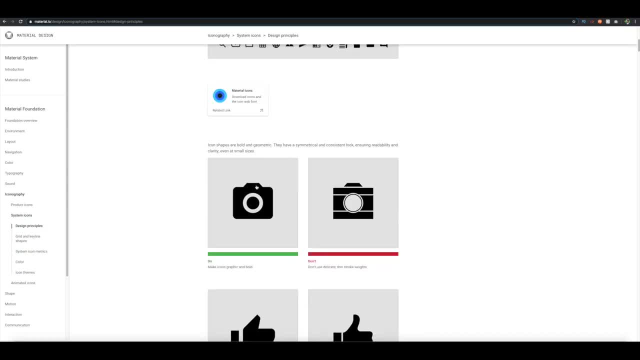 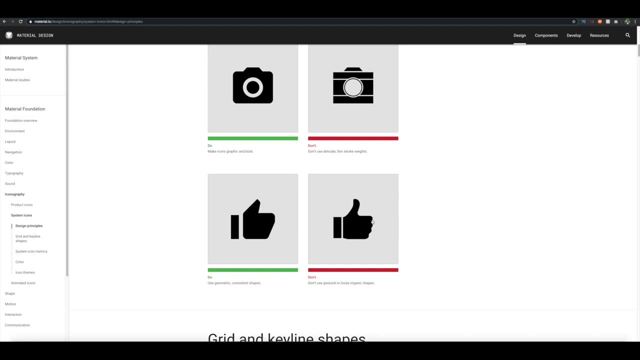 spending time making a shopping cart or something like that. if you don't want to making a shopping cart, Google have their own version of that, like here. they just have really simplistic ones. don't make it look like a form. make it look more geometric. a lot of this is basic shapes, basic geometry. other things to think. 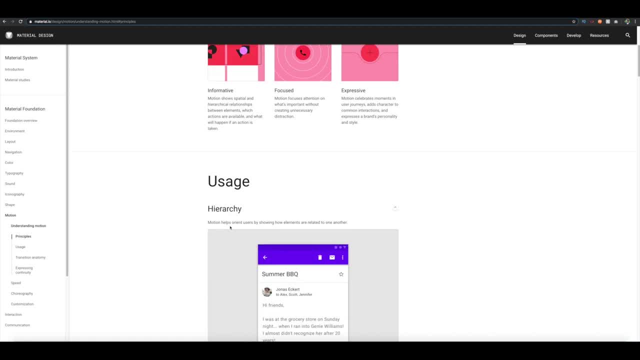 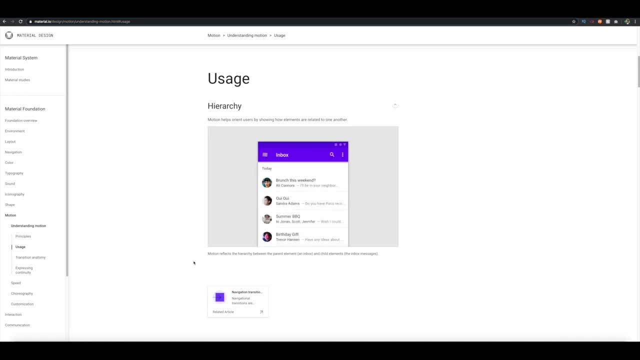 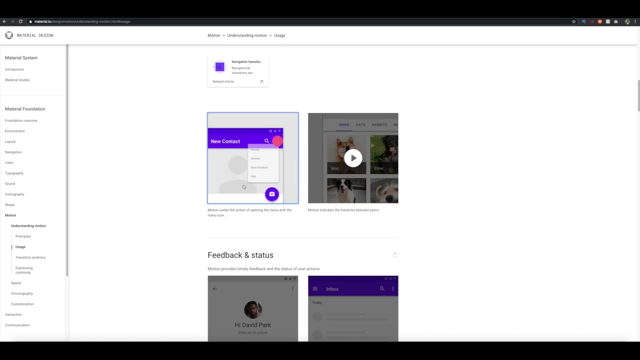 about is how motion is used. so some of the think about when you're designing these tools you can add motion and now? so maybe try and make it as realistic as possible so it helps your developers out. but you know they can't work magic. they have to work with the animations that 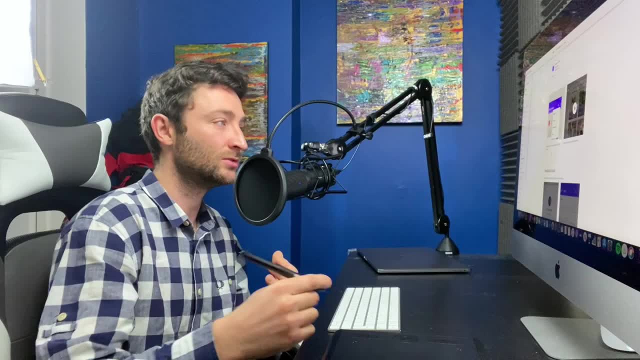 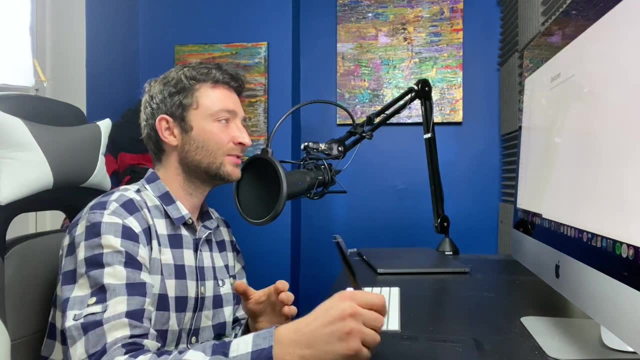 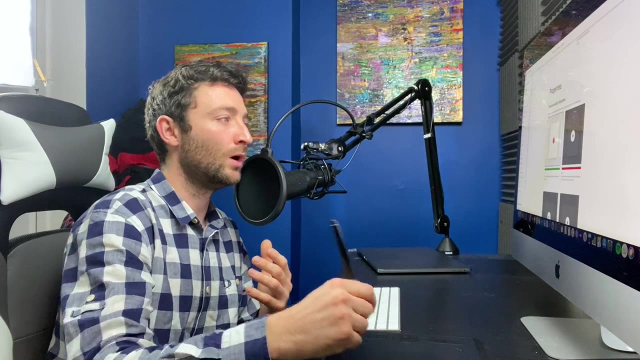 Android studio allows of them and as a designer, it's good to understand all of that by him by checking it, checking it out here. and then the last thing that they have on here is about interaction. so pinch and zoom gestures, what, what type of things to do? so they talk about what to do not do, so don't delay it, like. 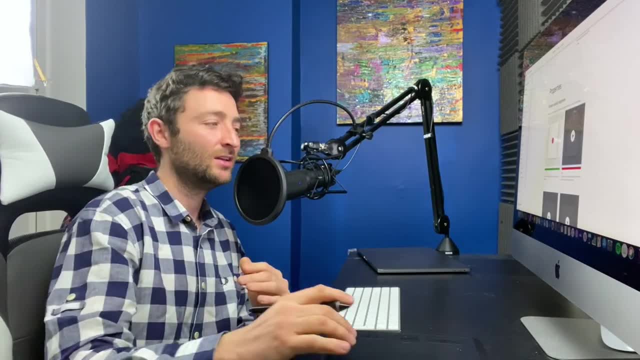 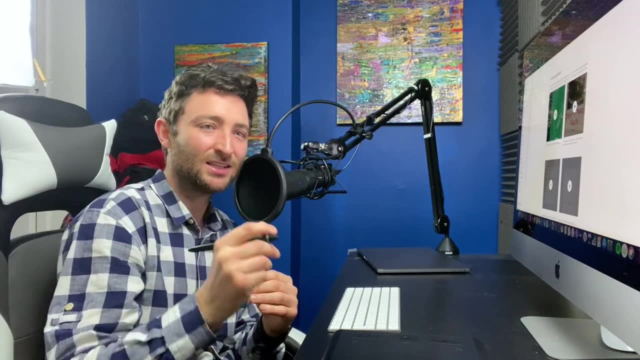 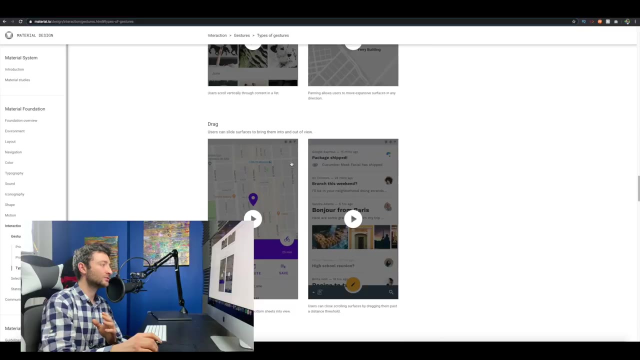 we've seen on a lot of these websites. now we're serving for an puzzle. need you around with a delay? it's something that I really I really don't like. they talk about indicating gestures, so little hides and stuff on a website. I think it's just if you're a designer, this is like a godsend. it's something that is an. 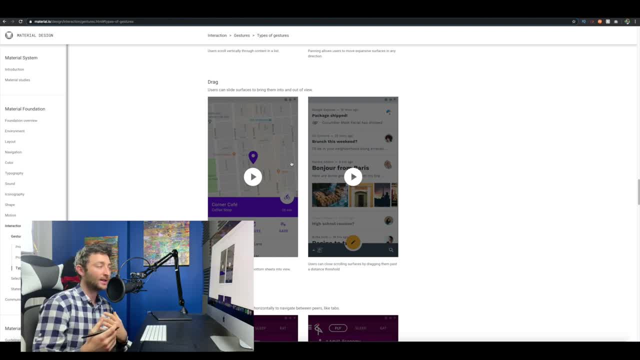 unreal resource for you. if I was designing for Android now, I would spend a whole day or a week learning this and then what I make at the end. it might take me a few hours to make, but compared to like spending a week messing around with it and half the stuff I won't be able to do anyway, I think that's a.